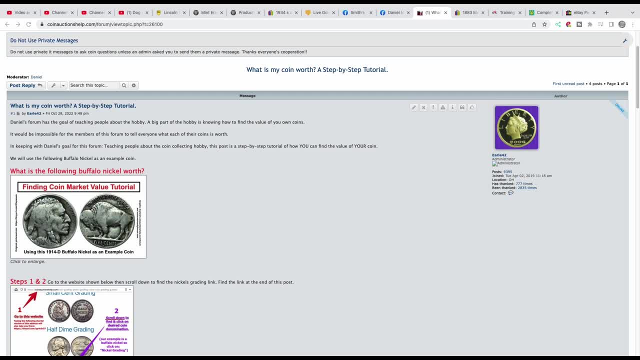 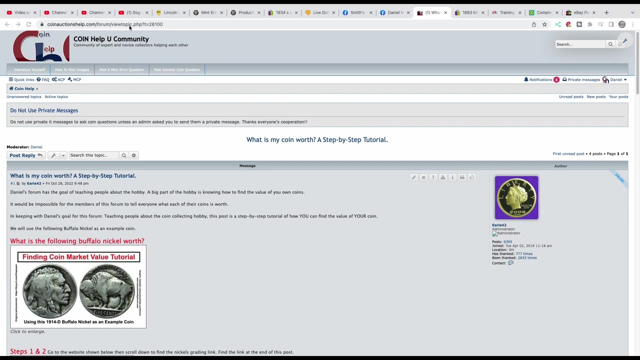 community in 2009, before I had my channel, And I get questions all the time on how much is my coin worth. Well, this is what you do. You can come over to the forum- and I do have links up here about posting images of your coin and asking questions, But you can actually just go to 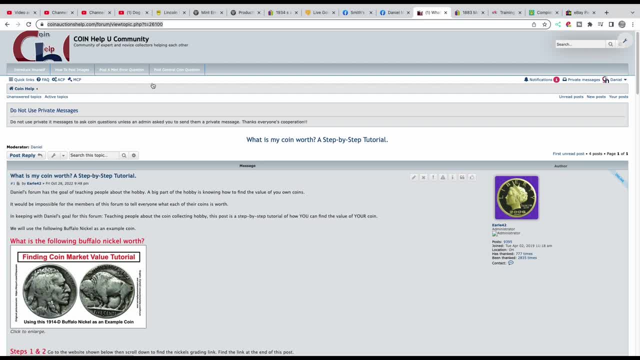 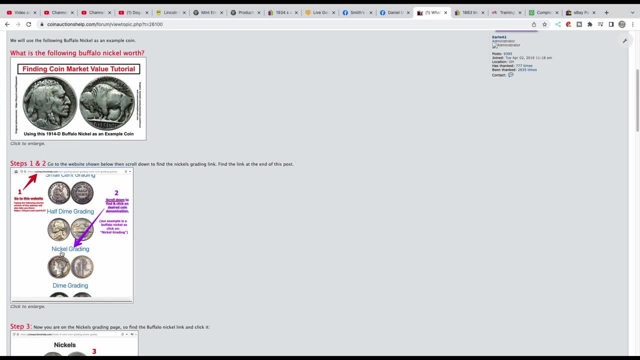 coinauctionshelpcom and I have a photo grade. So this is what we're looking at. So you've got this nickel right here. let's say So you've got this buffalo nickel. Then you want to go to my photo grade site. You want to click nickel grading right here. You'll go to my photo grade for the. 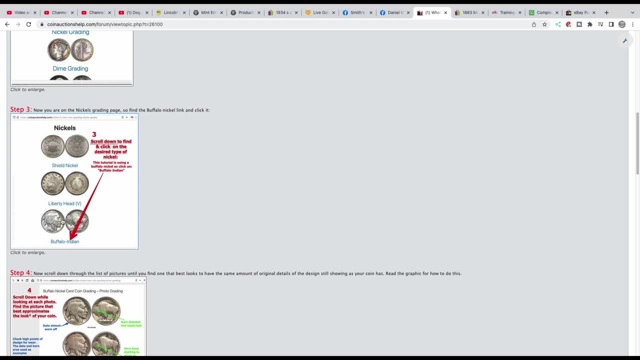 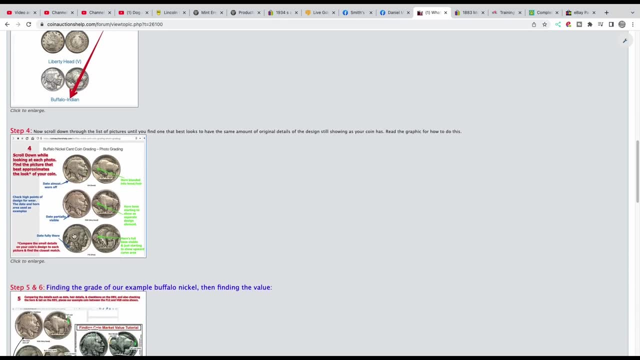 buffalo, Indian nickel, Okay, which is really a bison. So, anyways, you click on that and it will show you the different grades. Find the closest match you can find. You'll see the different matches you can find. Remember, you're just looking at a general idea of what your coin. 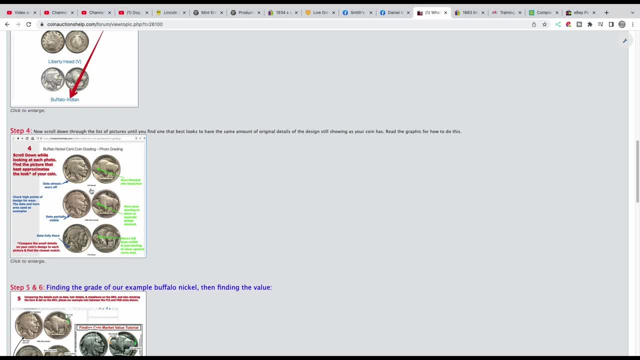 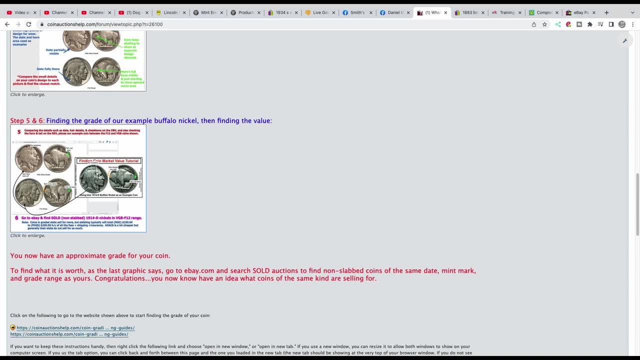 might look like compared to these images. Once you have it, it tells you very good, or g, or, or very fine, or fine. Once you find that okay, then you can go to a price guide or sold ebay auctions, Like you can buy a 2023 red book price guide. You can go to PCGS price guide, A numis media price guide. 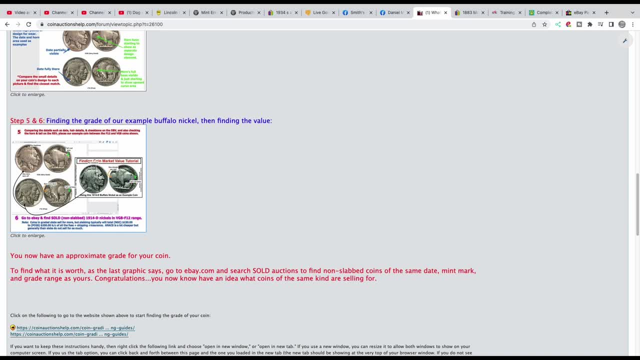 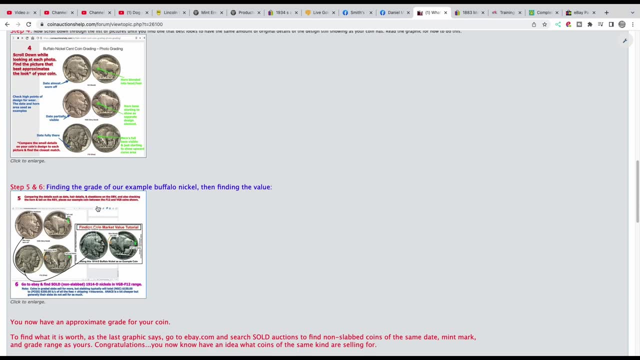 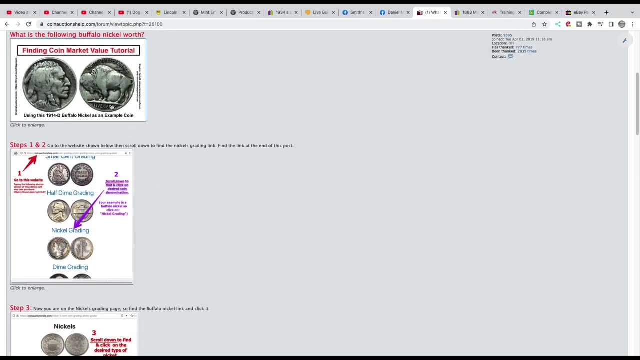 But always go to a price guide, not a google search. Look up the value for the grade you think your coin matches and all these images here right here. Once you do that, then you get an idea how much your coin is worth. You know a 14d is a little better date, So give it a shot. 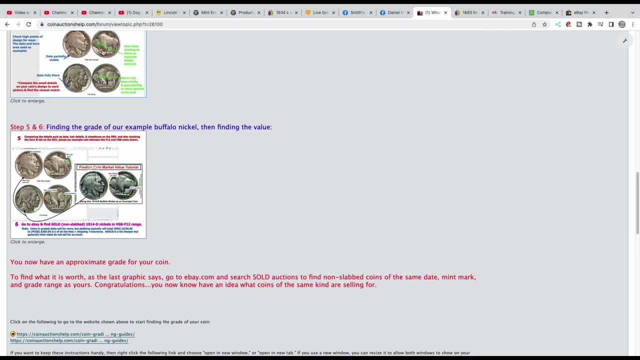 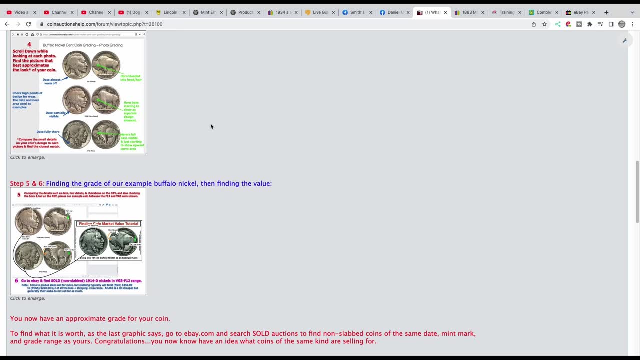 Try to match this over on my website with the photo grade here and then go to ebay and do a sold search, Do a little practice and guarantee you'll find out the value of your coins, and you will learn things in the meantime if you find anything else in the future. So thanks for. 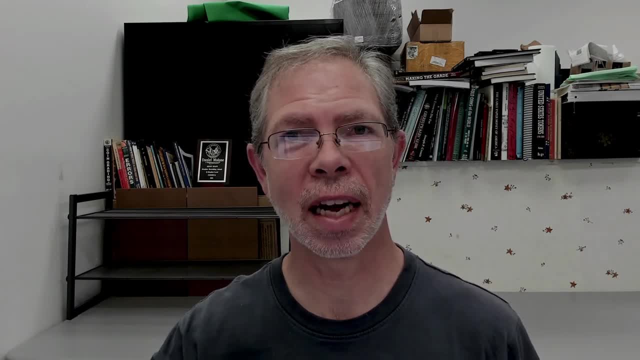 watching my latest video. Please like, share and comment And really share this, because a lot of people need to figure out how to find out their coin values instead of doing a google search. There's so many ads that point to Etsy and eBay, and 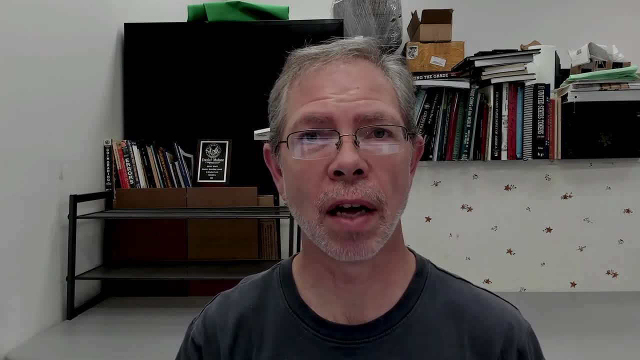 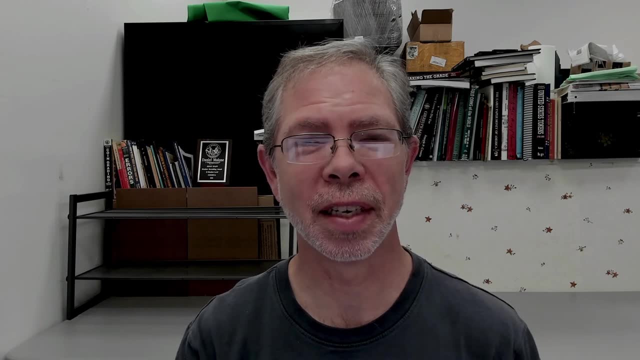 Bonanza and Mercanti that show coins being sold for thousands of dollars and they're not being sold. That's just what someone's trying to get out of them. So you want to find out the real coin values? follow the technique in this video. So with that, have a great day.